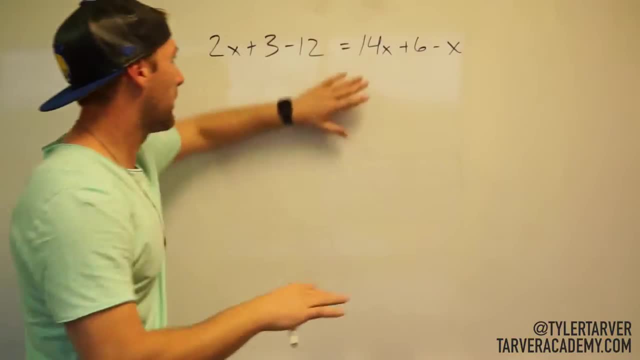 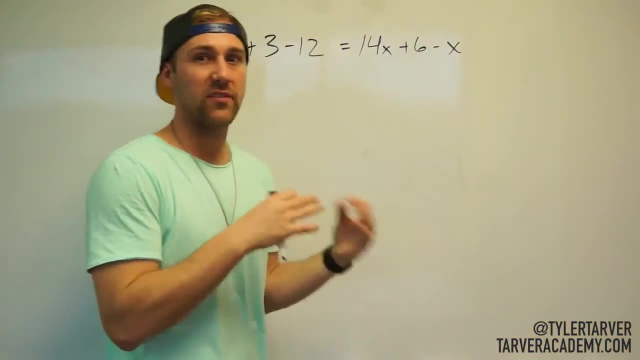 Color me right, Okay, So I'm going to let you pause it and then I'm going to show you how to work it. I want you to try it on your own first, because that helps you understand the problem more, Even if you get it wrong. it's good to try it yourself, because you can figure out where you 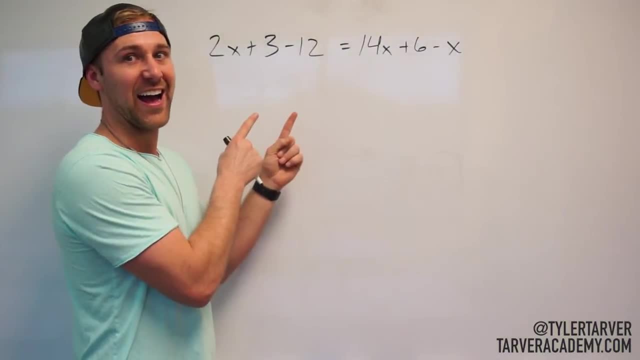 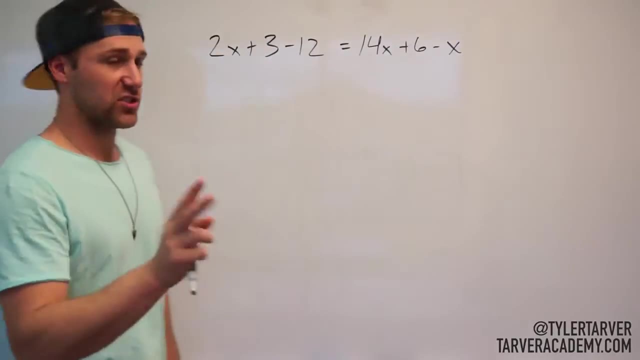 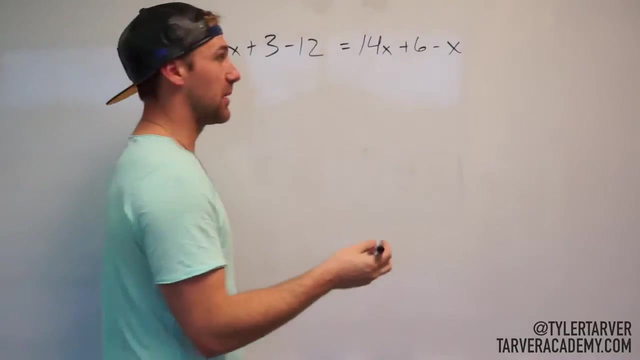 messed up. Ready, Pause it, write this down and give it a shot. Ready Go. Okay. So let's work this problem, shall we All right Now? there's essentially three steps. Let's say three, We'll find out if there's more. Okay, Whenever you're solving multi-step equation. All right, Do I have? 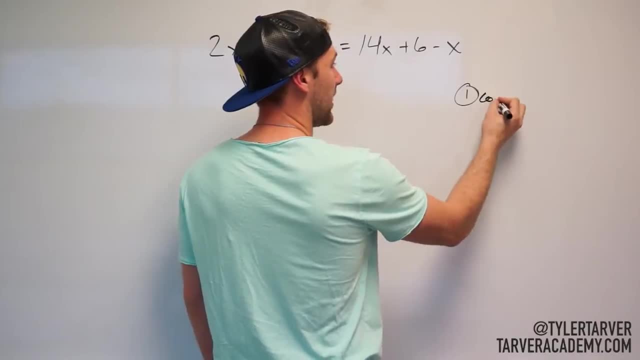 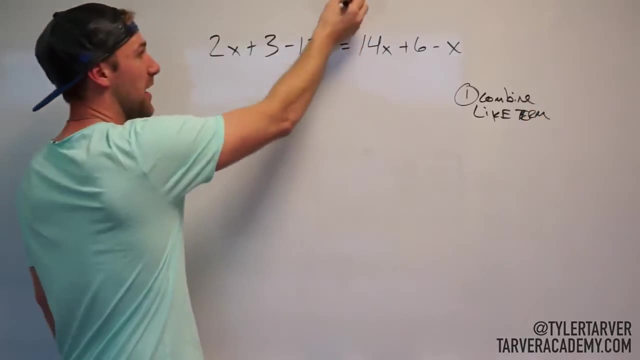 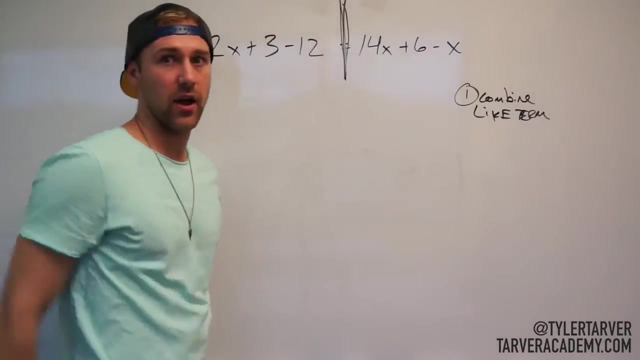 room over here. Yeah, First step, I want you to combine like terms, Like terms. That means I'm going to make a partition, I'm going to make a great wall right there between this side and this side. Okay, So what you want to do is you want to. 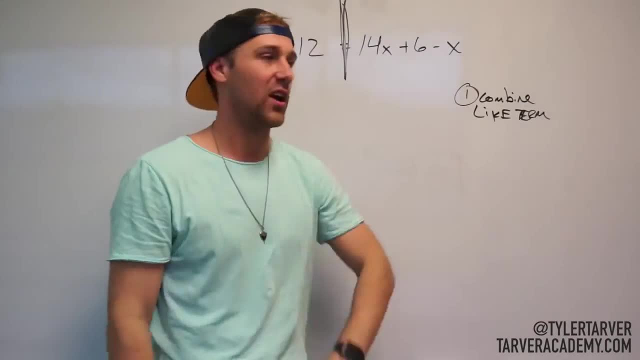 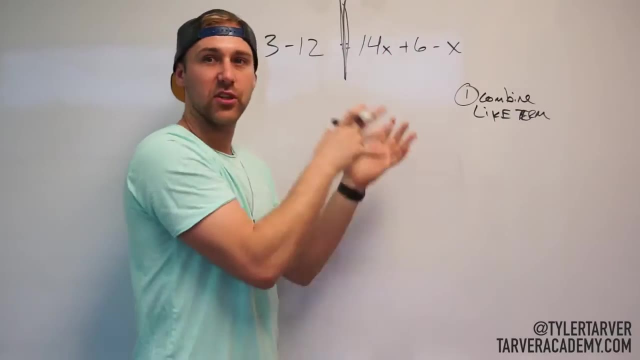 on one side. combine it like a regular math problem. Two plus two is four, Six plus two is eight. You know, four minus one is three. You want to do regular math, Regular math, regular math, until you make them as simple as possible. So that's combining like: 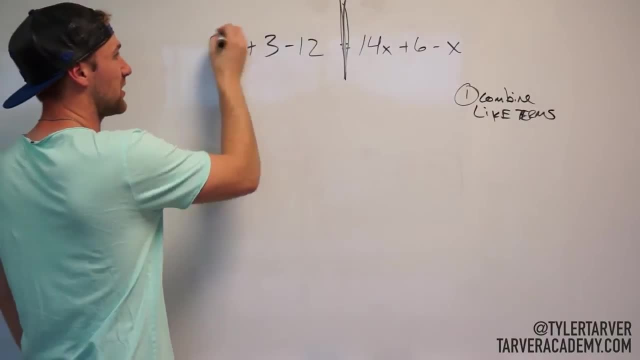 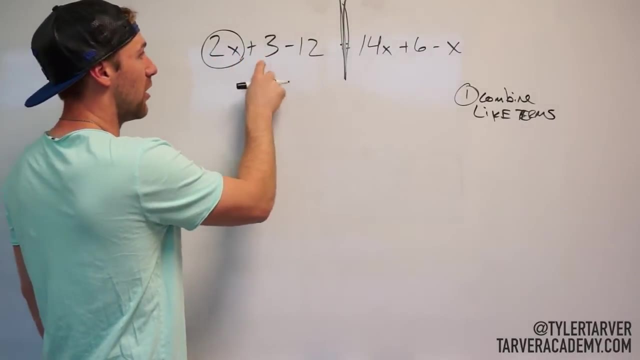 terms, So two X. I like to circle them because it makes me not skip anything. Can anything combine with two X? It has to have just one X with it for me to be able to. No, no, And I'm not crossing my. 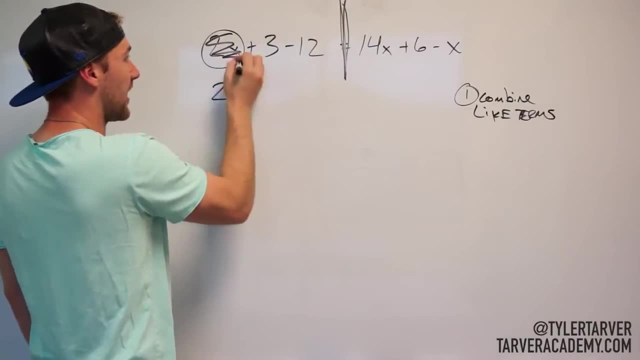 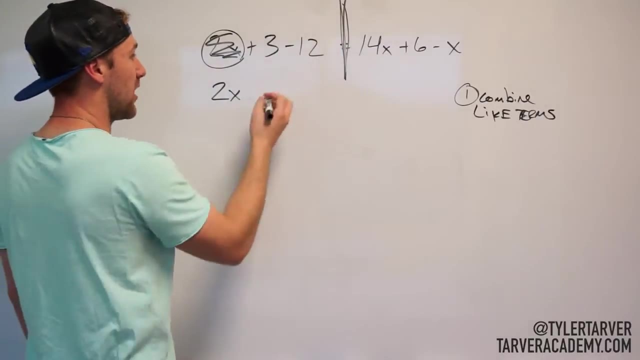 line yet. So two X is good. I'm bringing it down. Mark it out, so I know I've done it. Positive three minus 12.. That's a regular math equation. You can do that. You can do three minus 12, which would 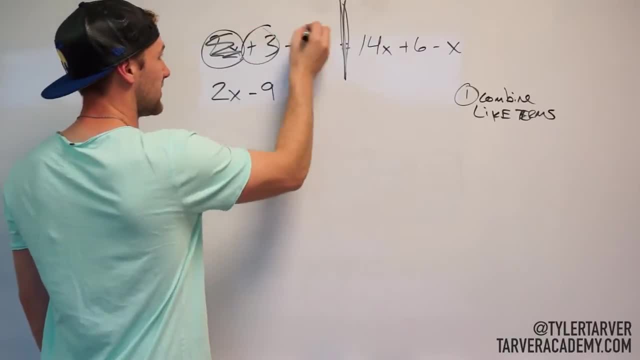 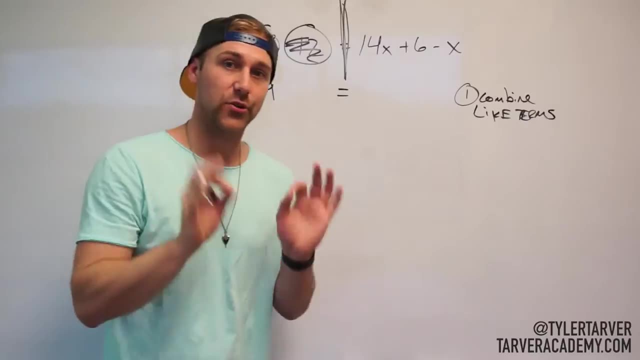 be negative nine. That's it. I've done this. I've done this. All my signs are included. I'm done. Bring down my equal sign. A lot of kids forget to bring down the equal sign. Do not forget. Don't be that kid. Bring down everything. Okay, Combining like terms over here, I'm going. 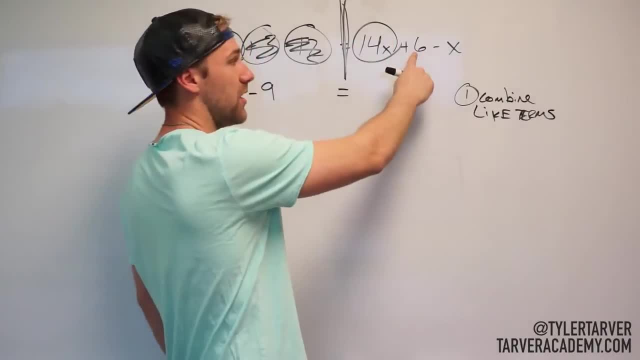 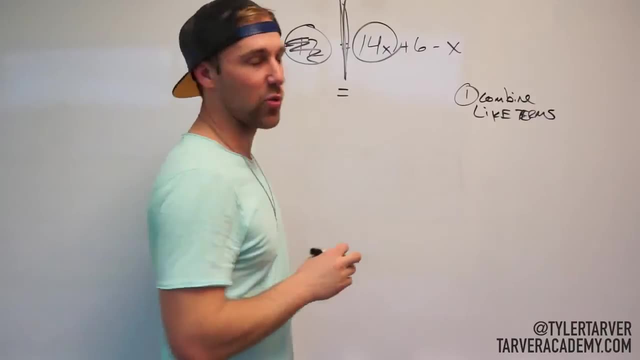 to start with my 14 X. Does that combine to 14 X? Negative ghost rider. Does 14 X minus X? does that combine- Yes, it does- to the greatest number in the world, 13, because 14 minus X. 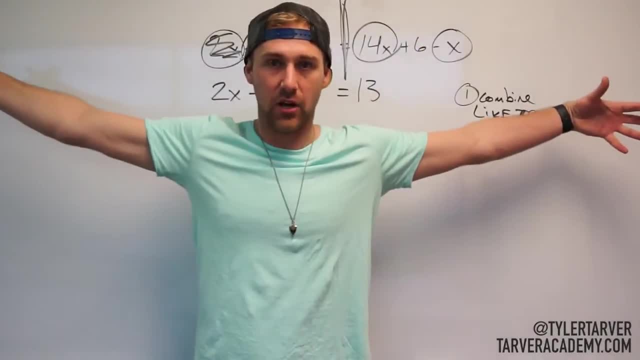 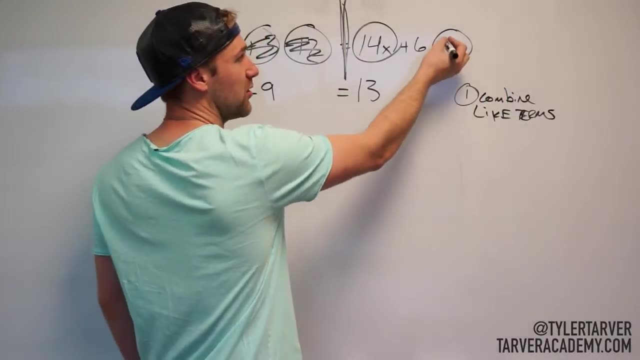 you're taking one of the X's. Imagine 14 X is lined up across in a line and you're taking one of them out, You're left with 13 X's. Okay, So we've got 14 X minus X, which also you always. 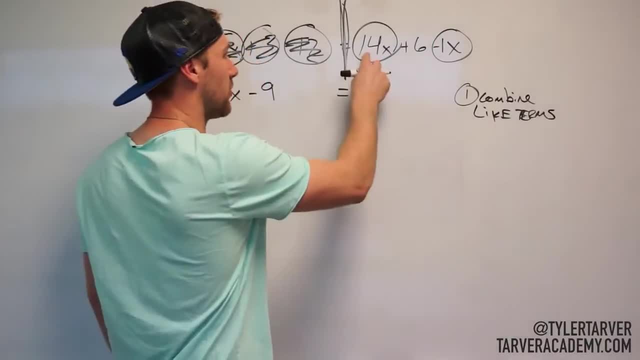 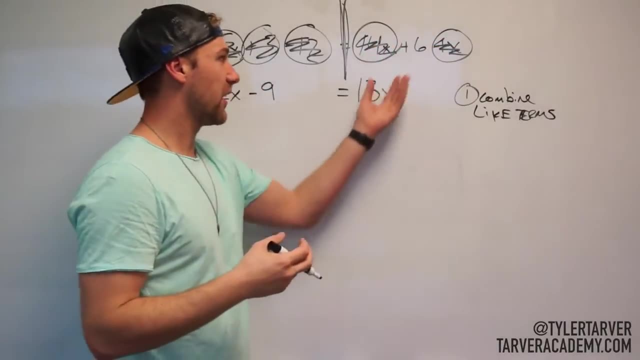 know that there's a one there, because anything times one is itself. So 14 X minus one X is 13 X. Another thing that students do a lot is they don't bring down like their X's. They get lazy or they get in a hurry and they just forget to bring down everything. Everything has to have. 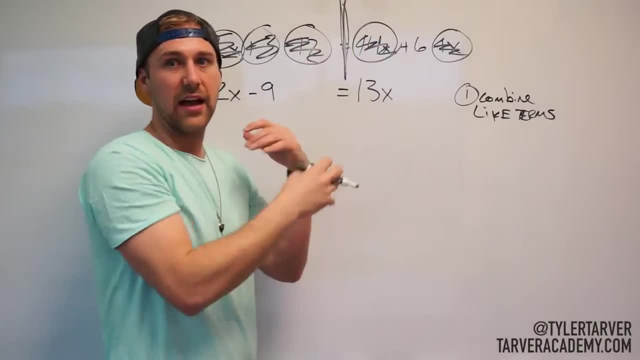 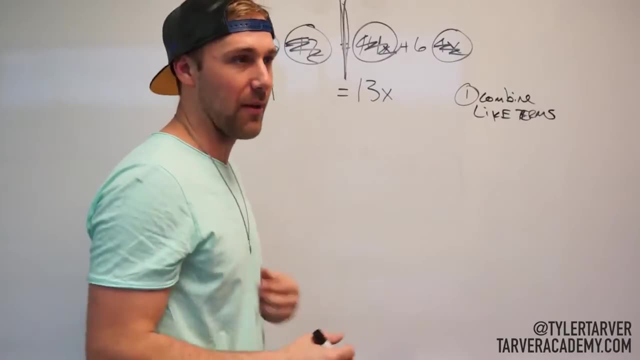 a reason for going away. I have to be combining or dividing. I have to be doing something to get rid of stuff. You can't just get rid of it because you don't want to write it anymore. That makes your math equation wrong. It doesn't work. in math History, apparently they can cut. 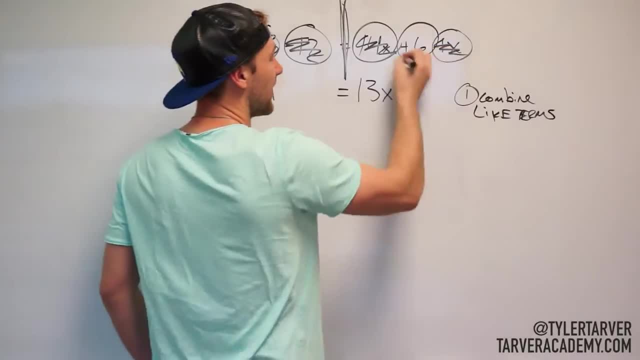 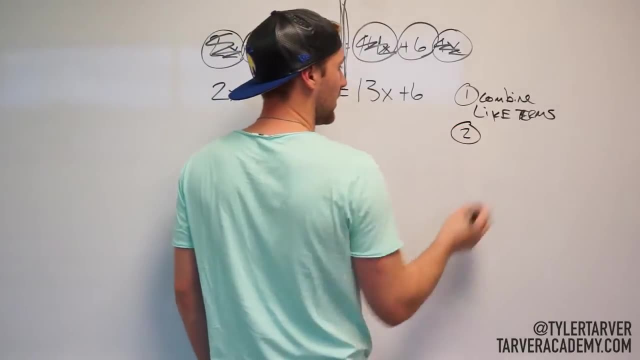 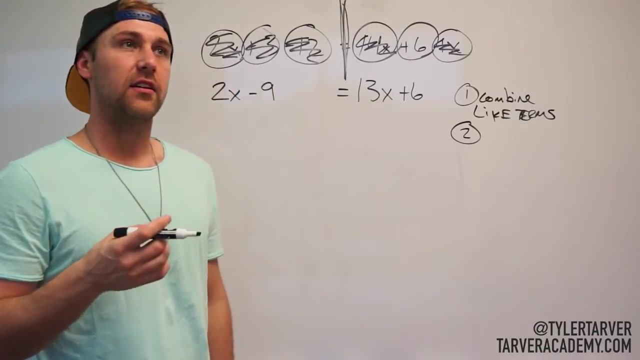 out whatever they want from history Math. you have to leave it in there, Okay, And there's nothing left to combine with that. So it's plus six. Okay, I combine my like terms. Next step: I'm trying to think of the best way to word this. Best way to word this is get X by itself, Let's. 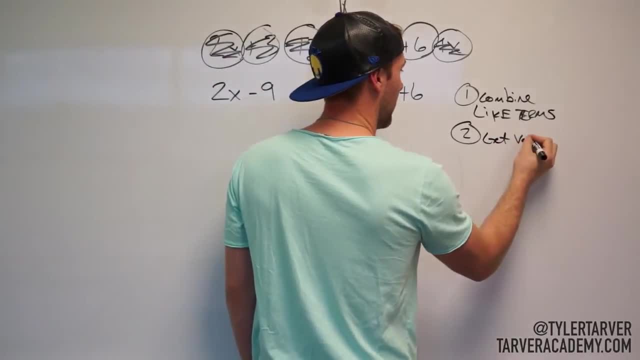 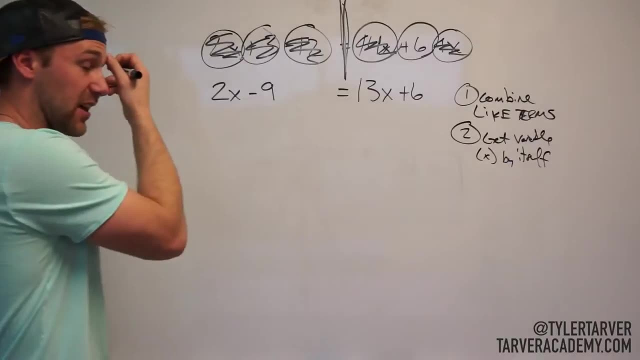 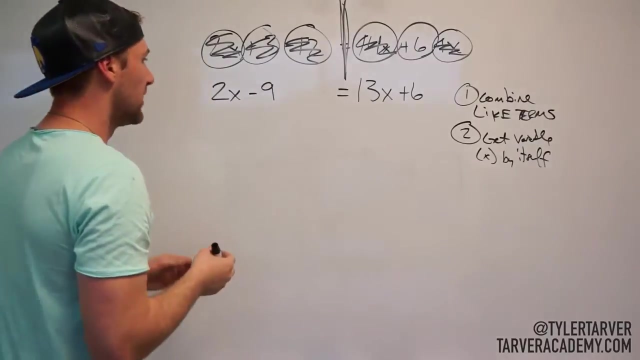 say that: Or get the variable by itself, Get variable. In this case it's X, Get the variable by itself. To do that, you've got to get all your X's to one side and all your regular numbers to one side. Okay, So let's say we've got a bigger amount of X's over here, So 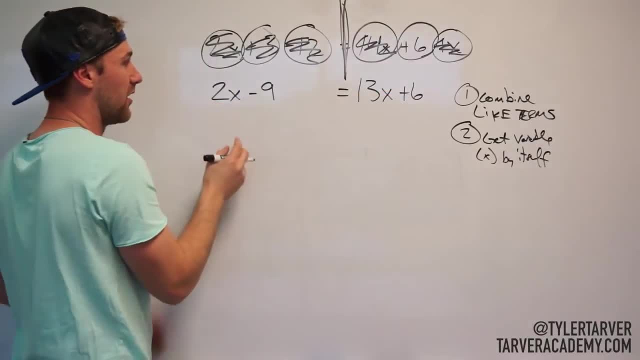 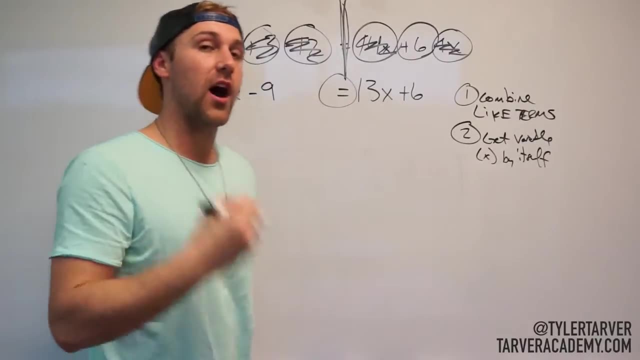 I want to get these X's over here. I want to get these regular numbers over here. Okay, So now that you're going across the equal sign, you're going to have to do the opposites. This is a positive 2X. 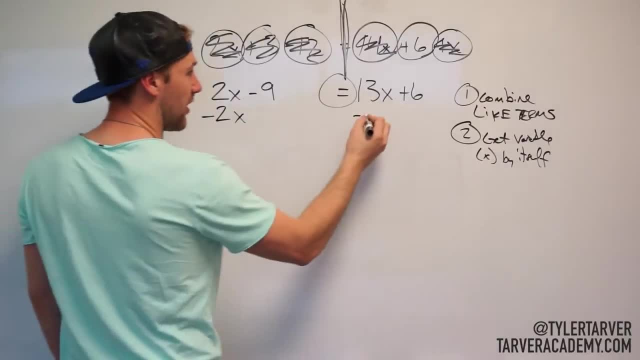 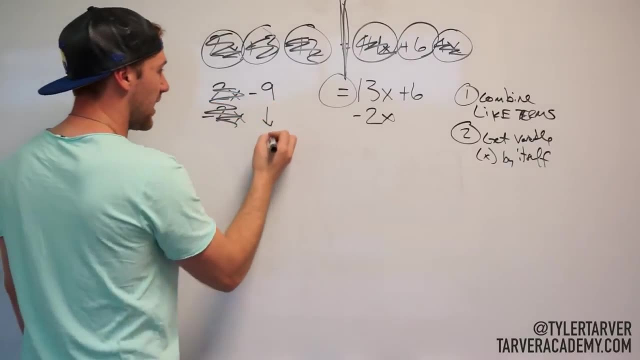 Opposite of positive 2X Subtract 2X. I have to do that from both sides, If not I'm breaking math law. 2X minus 2X is zero, So that goes away. I bring down my negative nine. I bring down my equal sign: 13X minus 2X, 13 minus. 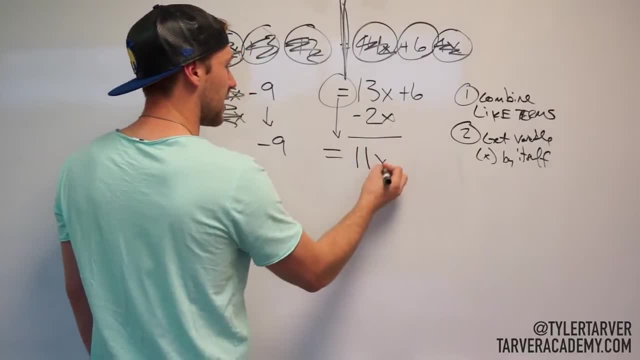 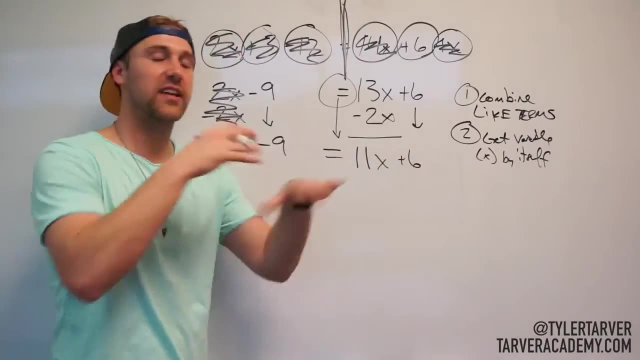 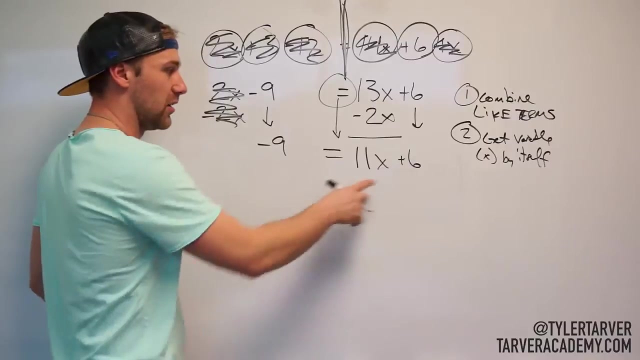 two is 11X, And then I'm going to bring down the six, because we're just not there yet. Plus six. Everything's been brought down, Everything's accounted for. Okay, Now I got my X's and my X's over here. Now I need to get my regular numbers over here. Regular number over here is: 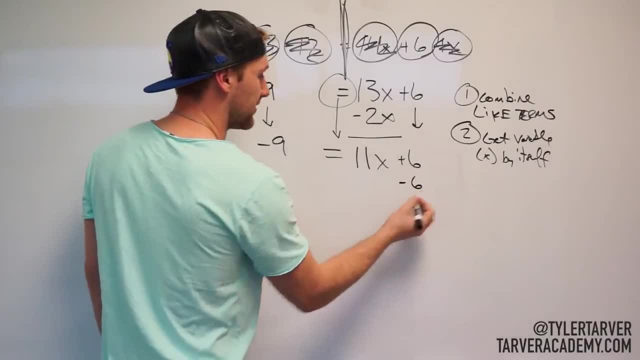 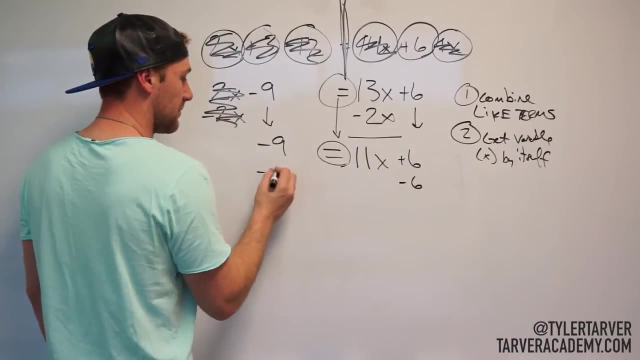 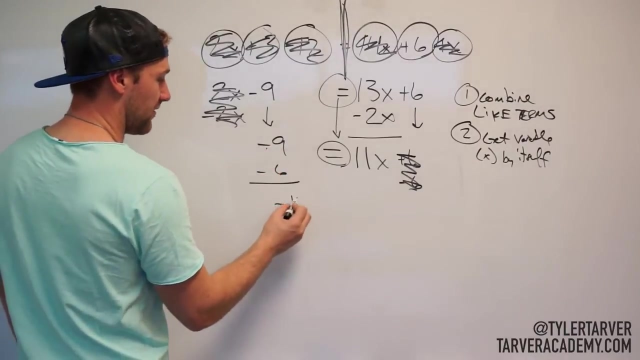 positive six, The opposite of positive six, Negative six. Why am I doing the opposite? Because it's going across the equal sign, So I got to do opposites: Positive six minus six Minus six. That becomes zero and cancels out. Negative nine minus six, Negative 15.. Okay, It becomes a.